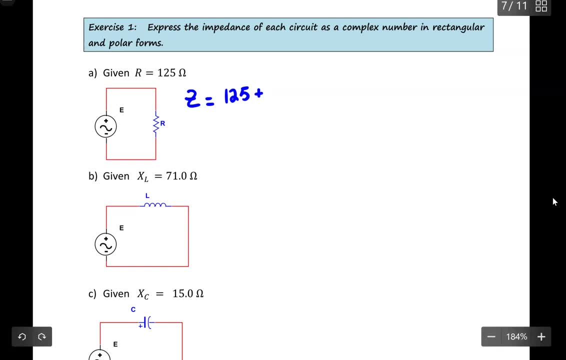 And I strongly recommend that everyone write 0J. So use your calculator. Casio FX, And a few simple keys on that calculator will convert this complex number from rectangular to polar form, And it's actually equal to 125.. And the angle is 0 degrees And both measure in ohms. So keep that in mind. 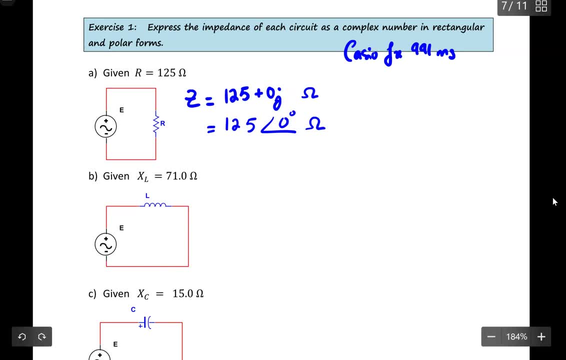 Okay. So if you want to, If you want to visualize this in terms of the phasor diagram and you don't need to use a calculator to convert between rectangular and polar, then we can review it as this. Okay, So I draw a complex plane. This is the real part And this is the imaginary axis. 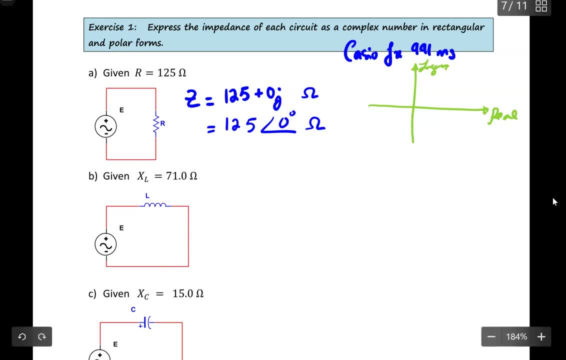 Okay, So on this real axis, I will project on this the vector for the resistor, which is equal to 125.. So if you go from the origin to here, let's say this is equal to R, equal to 125 ohms. 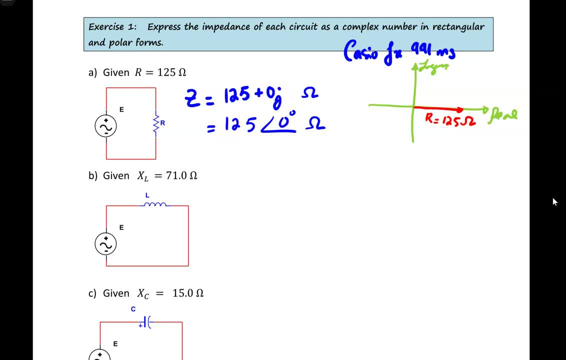 Okay, So the value of the resistor will always take the positive x-axis or the positive real axis of this complex plane. So, as you see, in polar form it would be a 0. Number of degrees angle in this case. Okay. However, it's a good idea to review and also to key into your calculator to figure out the answer for this. 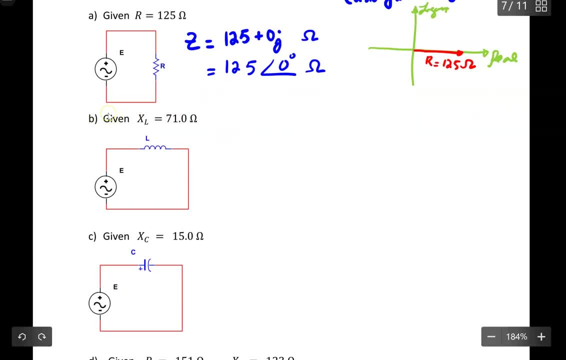 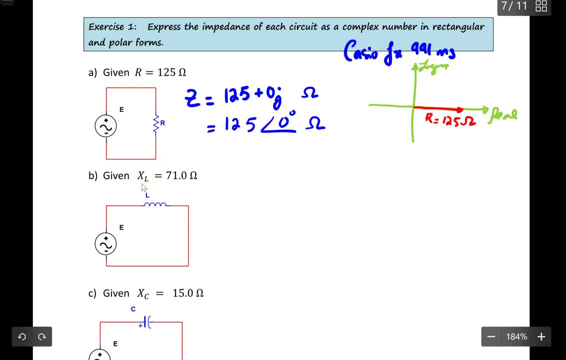 Okay. So if we go to question number B, Okay, Don't forget that I am giving everyone the value as the reactants. Okay, So we can use the reactants. Okay, So we can use the reactants to write our impedance in both rectangular and in polar form. we don't. 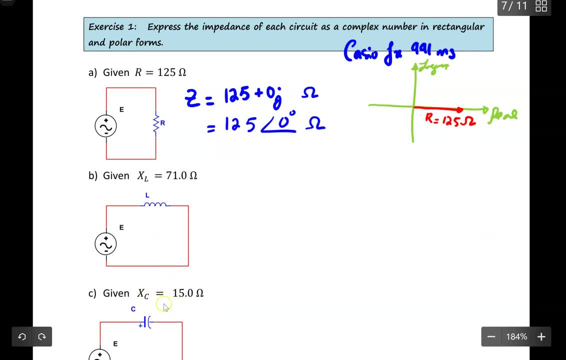 have to calculate this value right here is already given to us as the reactants. okay, so for question number B: okay, in this circuit I only connect the inductor in this case, so Z will be equal to. okay, I don't have a resistor, so the real part. 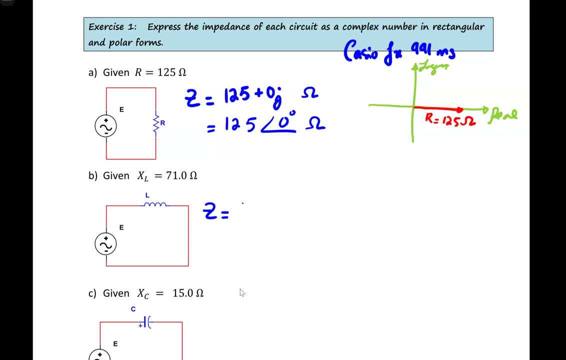 of this complex number in rectangular form would be equal to zero, and XL takes on the positive part of J, so I would write plus seventy one point zero, minus J. alright, okay, so if you visualize this on the complex plane, okay, again, this is real, this is imaginary, okay, and I have my XL represented as such. okay, so this? 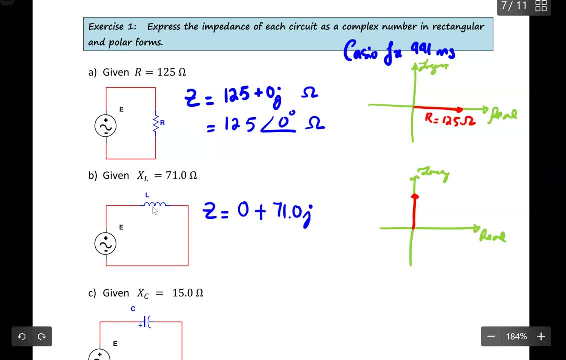 is my XL and is a plus 71 J in this, okay, and is a plus 71 J in this- okay, and is a plus 71 J in this case. and if you take a look at this diagram, you can see that the angle would be equal to 90 degrees, okay. so, at the same time, if you use your calculator and 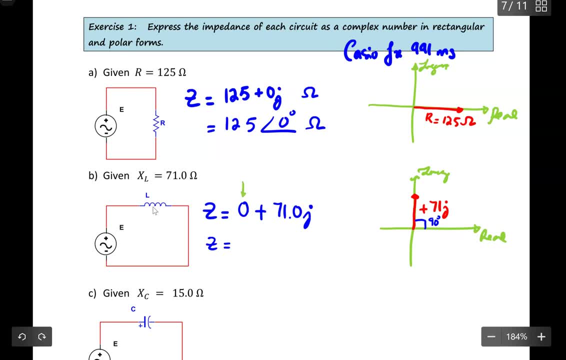 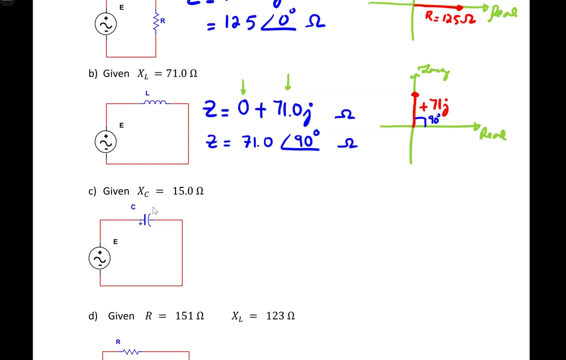 you key this value into your calculator as the real part, this value into your calculator as the imaginary part, then your answer would be 71.0 and the angle expressed as 90 degrees angles. again, both measure in ohms. all right, okay, so what about for C? for C, what I have in this case is I connect it with just a. 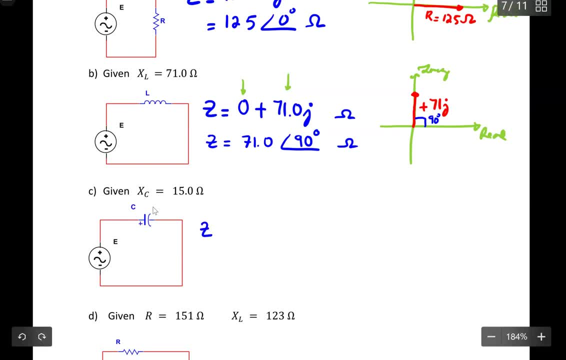 capacitor. okay so. so what about for C for C? what I have in this case is I connect it with just a. So what about for C for C? what I have in this case is I connect it with just a. Z is equal to zero, because I don't have a resistor in this case, but I will. 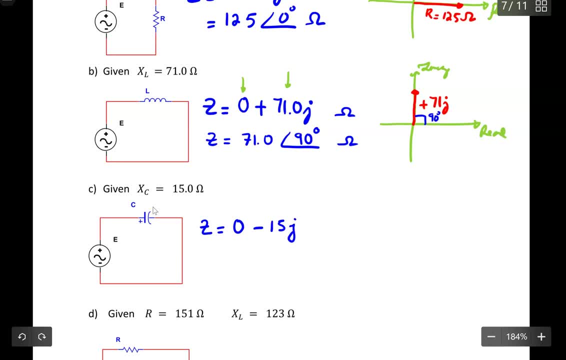 subtract that with 15 J's. ohm, why is it negative? 15 J is because the capacitive reactance will take a negative part of J on the complex plane. so to visualize that, or to draw the phasor diagram, that, or to draw the phasor diagram, and again we are going to label our axis. 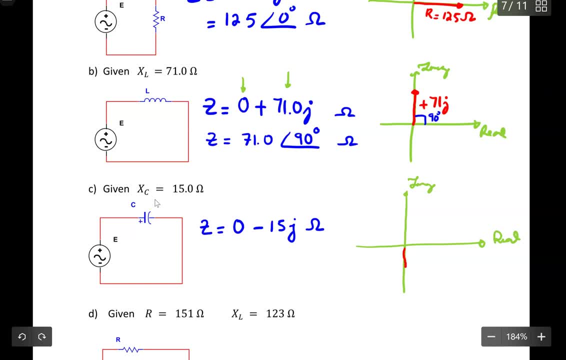 and again we are going to label our axis, and again we are going to label our axis and I can present this one as it's going, and I can present this one as it's going, and I can present this one as it's going down to this part. so it's negative: 15 J. 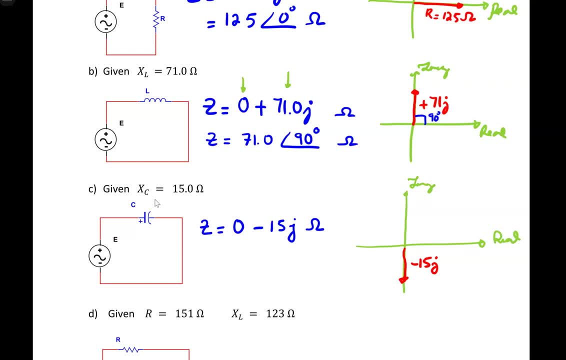 down to this part, so it's negative: 15 J down to this part. so it's negative: 15 J in this case. all right, okay. so if we are in this case all right, okay, so, if we are in this case all right, okay. so if we are talking about the angle or the argument, 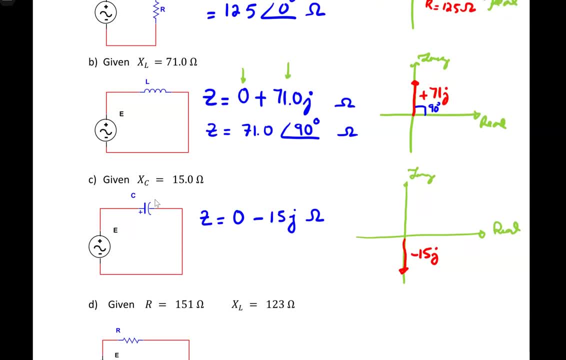 talking about the angle or the argument, talking about the angle or the argument in this case, then we are talking about: in this case, then we are talking about: in this case, then we are talking about this angle right here, which is represented, this angle right here, which is represented. 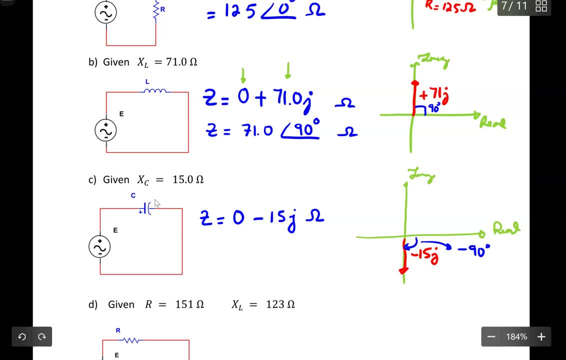 as negative 90 degrees, or we can talk about this angle as counterclockwise, which should be equal to 270 degrees. Okay, so, if you use your calculator, your calculator will give you the following values in term of polar form, So it will be 15.0. 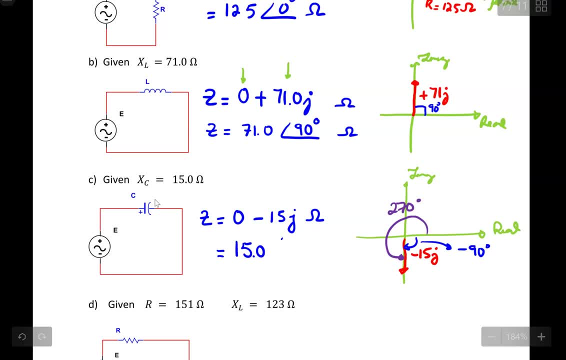 as the modulus and the argument will be equal to negative 90.0 degrees. Again, I try to express this as complex number in three significant digits. Okay, so this is equivalent to 15.0 and 270 degrees as three significant digits. Okay, so then I should put 15.0. 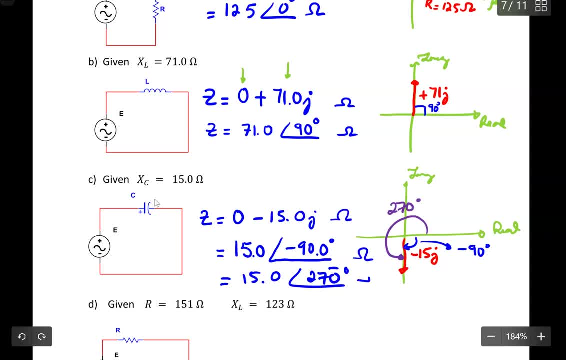 j here, so that I can express this as three significant digits as well. Okay, so don't forget the angles. Okay, the angle: if you go clockwise, you will have a negative angle. If you go counterclockwise, you have a positive angle. So, in this case, 270 degrees. 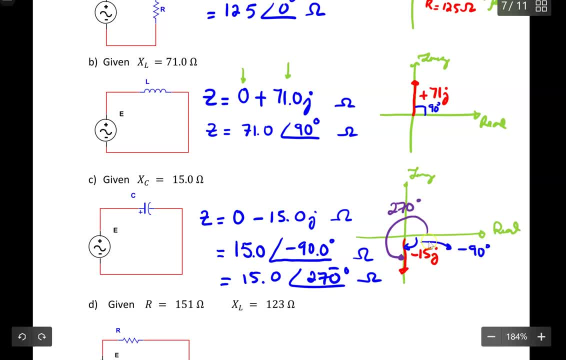 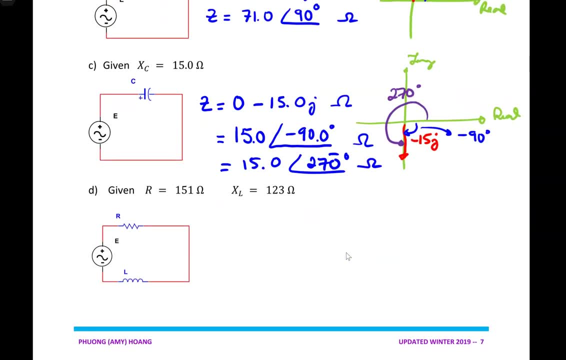 is equivalent to a negative 90 degrees for the argument for this complex number in polar form. Okay, so let's go over the d, Excuse me. So for d z will be equal to 151 as real, plus 113 j in ohms. 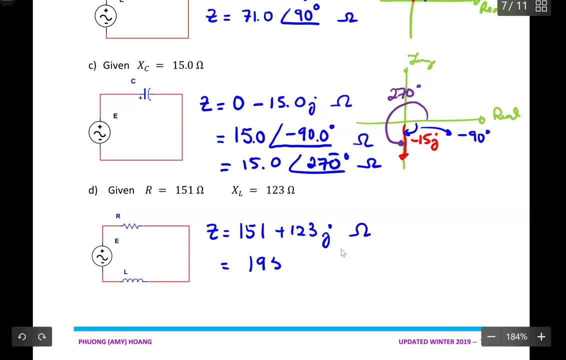 Convert to polar, I should have it as 195 and the angle as 39.2 degrees ohms. Okay, so now let's go over the d, Excuse me. So for d z will be equal to 151 as real, plus 113 j in ohms. Convert to polar, I should have it as 195 and the angle as 39.2 degrees ohms. 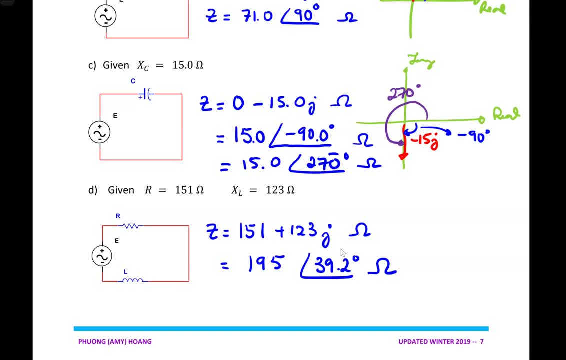 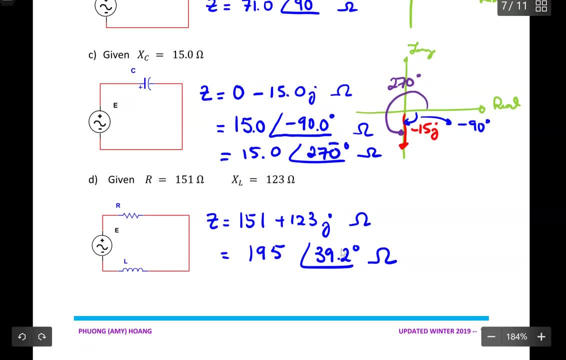 Okay, so now let's go over. the d. z will be equal to 151 as real, plus 113 j in ohms. Convert to polar I should have it as 35.2 degrees ohms. So this is the ough. So let's move on to the next example. 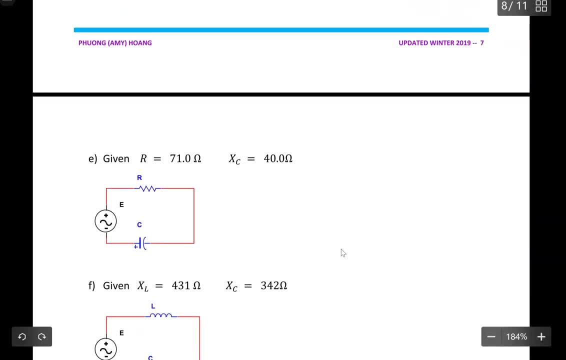 this is the next example, which is this diagram e. So in here I have xz, the capacitive reactants and the resistor. So to find z, I will write z is equal to 171. So to find z, I will write z is equal to 171. 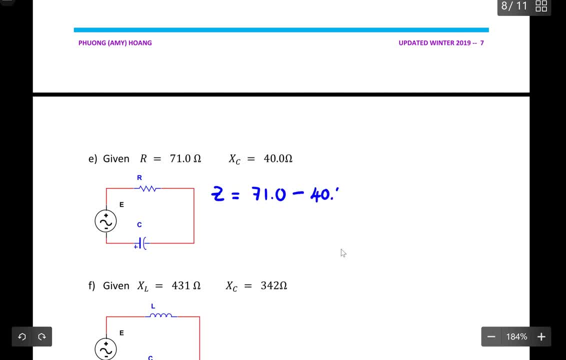 And I subtract this with 40.0 J because the capacitive reactants will take the negative part of J. Then, to present this as polar form, I will have it 81.5 and the angles as negative 29.4 degrees. 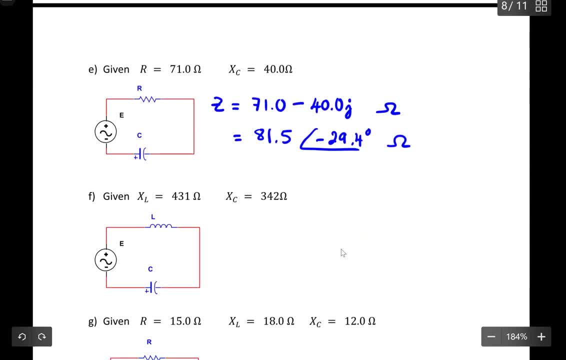 So again, they measure in ohms. So let's quickly go over this. I have F, So for F, I don't have a resistor in this case, but I am given the values for xL and the values for xC. 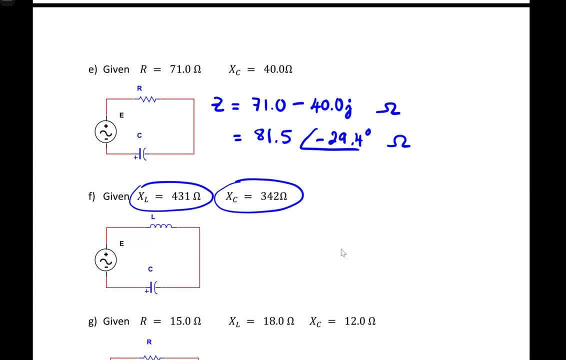 Okay, so how do I write the complex number in rectangular form? So I would like everyone to recall this formula that I have shown Everyone, Everyone- from previous lesson: the reactants, in term of magnitude, will be equal to the xL subtract the xC always. 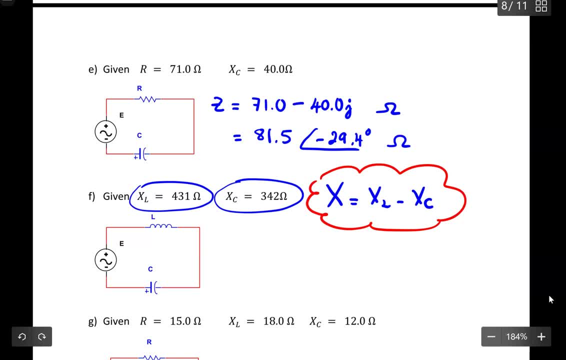 Alright, So keep this formula in mind. Then the first thing I do is I will find x. by taking xL subtract xC, I will have 431.. Subtract Subtract 342.. So I will have it as 81.. 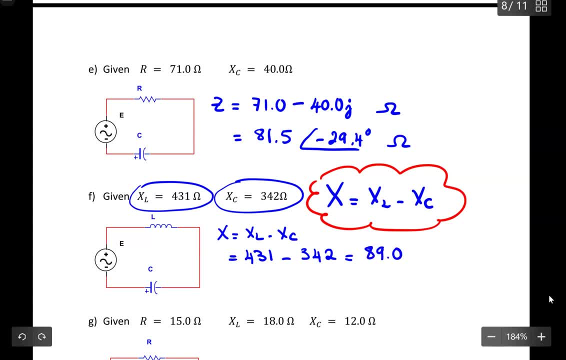 I mean 89.0.. Okay, So this number turns out to be a positive number. So you use that exact positive number to put it into your complex number. You put the x in rectangular form, So in this case I don't have a resistor. 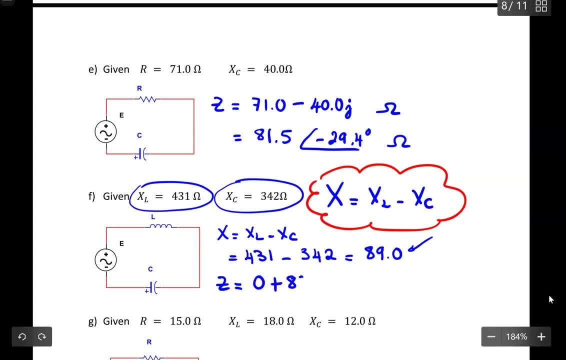 So it's a zero. And you add that with 89.0 j And using your calculator, convert this into polar form. Again it will be 89.0.. And you see, Right away you can recognize that the angle is equal to 90 degrees. 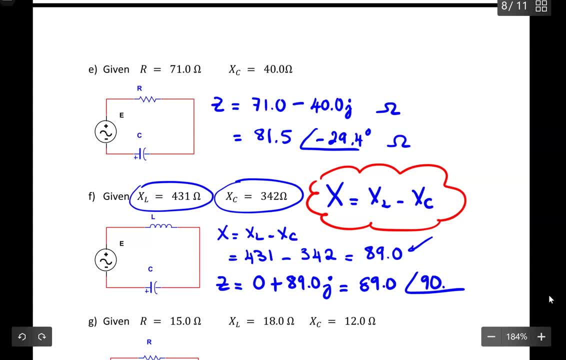 Okay, So they all measure in ohms. So if I have this, this will be equal to the angle. So if I have this, this is the energy, And you add this here, Then I can write down the result out. 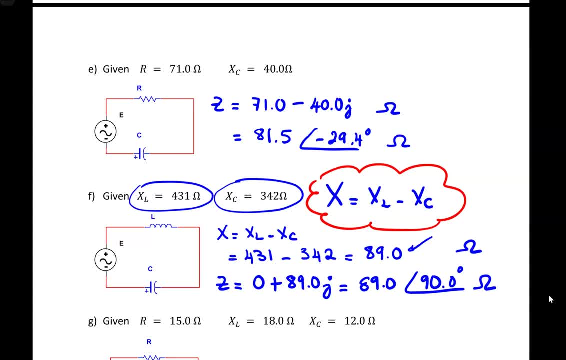 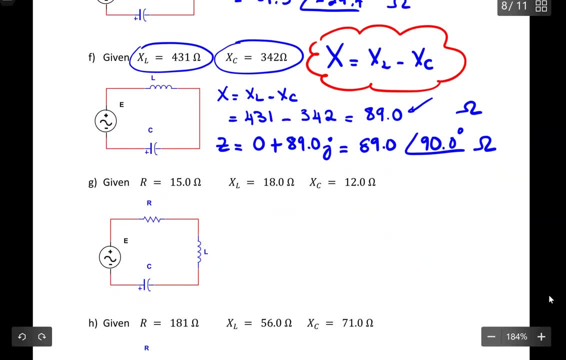 Okay, So this is the angular mass And that is the vector mass, The body mass that is equal to the angular mass. Okay, it's quite important and keep that in mind. okay, so for number J, okay again, I will calculate X by taking the XL subtract the XC, so I will have 18. 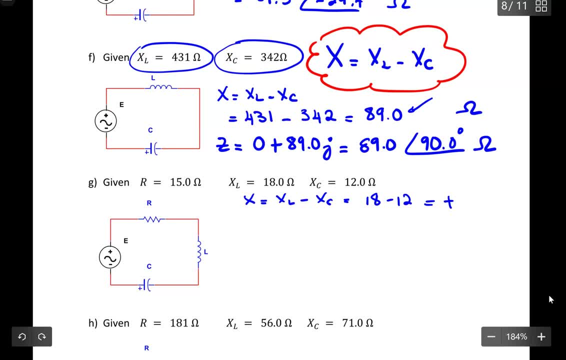 subtract 12, so I will have it as positive 6. okay, so Z will be equal to 2. the R is given as 15.0. I add that with 6.00 J ohms, convert this to polar, it should be equal to 16.2 and the argument turns into 21.8. 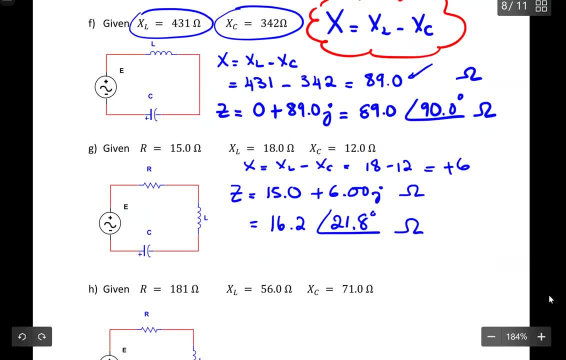 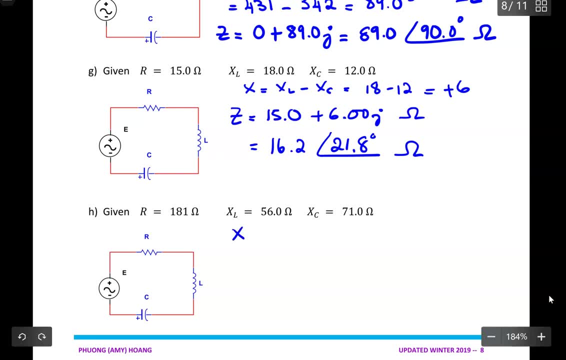 degrees and measures in ohms. all right, what about H? so in H again, I will have to calculate the reactants. in H, again, I will have to calculate the reactants by taking the inductive reactants subtract the capacitive reactants. so I will have 56 subtract 71, 56 subtract 71. excuse me, my answer is equal to a.